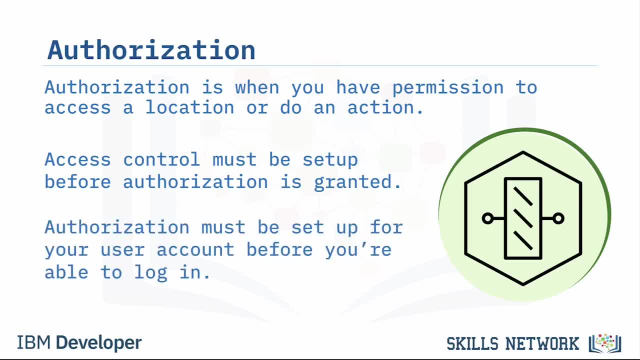 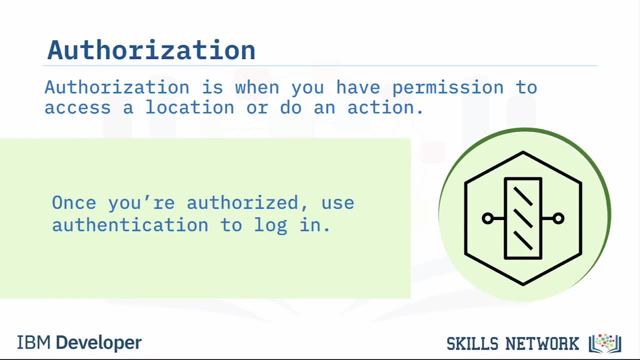 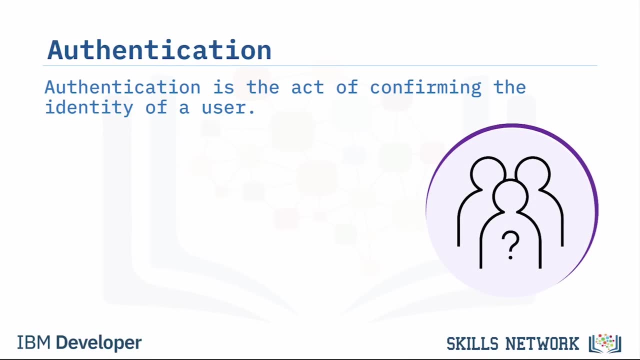 maintain data security, and authorization must be set up for your user account before to log in. Once you are authorized, you can then use authentication to log in. Authentication is the act of confirming the identity of a user. Authentication involves two steps: entering the correct login information and confirming that it is really you. Authentication: 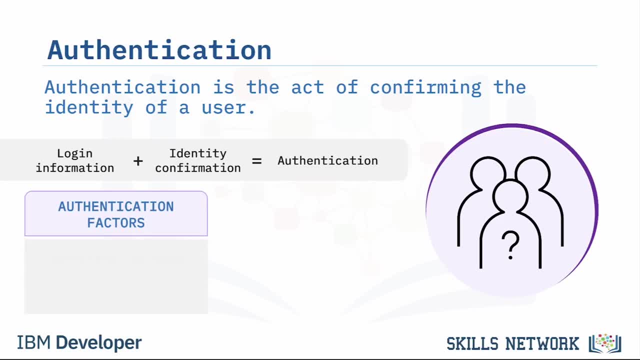 factors used to confirm identity include something you know, like a username, password, PIN or answers to security questions. Something you have, like a mobile device security key or security badge, And something you are- biometrics, like facial recognition or a fingerprint. 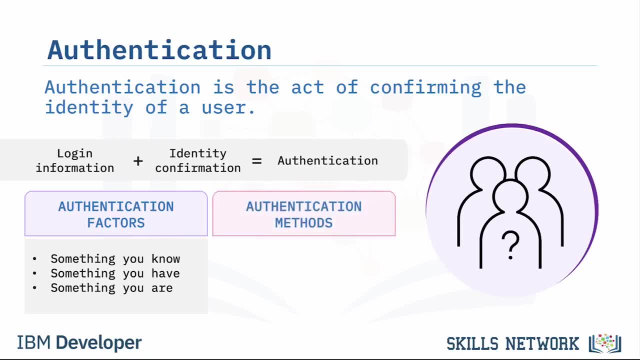 iris or voice scan. Authentication methods include single factor or SFA, two factor or 2FA, multi-factor or MFA and single sign-on or SSO. SSO lets you log in to multiple devices, such as a mobile device or a security key or a security badge. 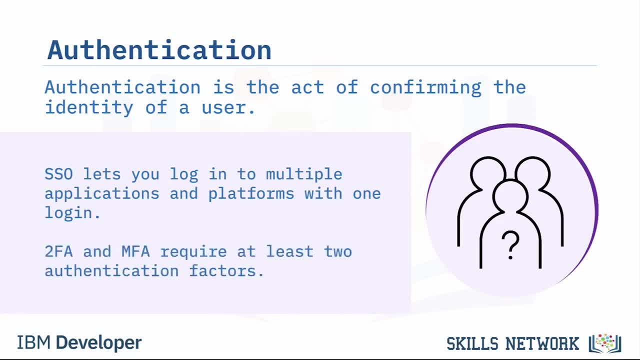 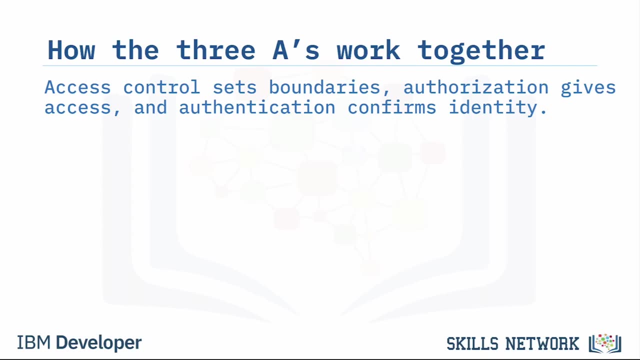 SSO lets you log in to multiple applications and platforms with one login. 2FA and MFA are the most secure ways to log in because they require at least two authentication factors: Access control sets boundaries, authorization gives access and authentication confirms identity. In the security field, it's important to know the right balance between the three A's. 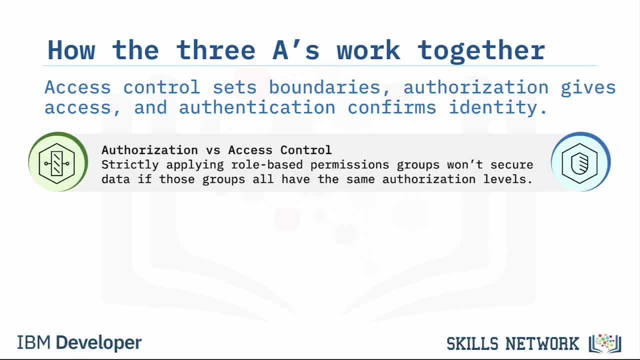 Strictly applying role-based permissions groups won't secure data if those groups all have the same authorization levels. The same is true if groups have properly set permissions but are not properly applied by administrators. Using strong passwords and MFA won't secure data. if all groups have the same permissions, The same problem exists if groups 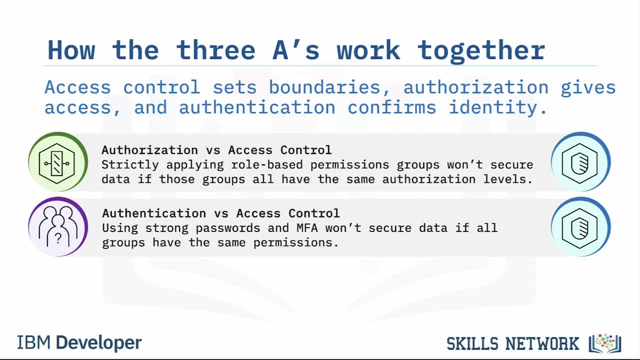 have properly set permissions, but passwords are weak. Using strong passwords and MFA won't secure data if all users are assigned to the same group, The same problem exists if administrators assign users to the proper groups, but passwords are weak. Best practice should require strong authentication, strong authorization and strong 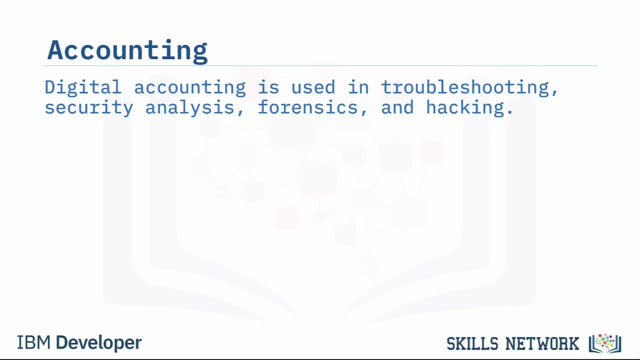 access control. Digital accounting is used in troubleshooting, security analysis, forensics and hacking Logs. Most software and systems generate audit logs. Audit logs capture log file. events Logs can show who did what and how the system behaved. Tracking Websites can track your OS browser version, installed extensions. screen resolution. 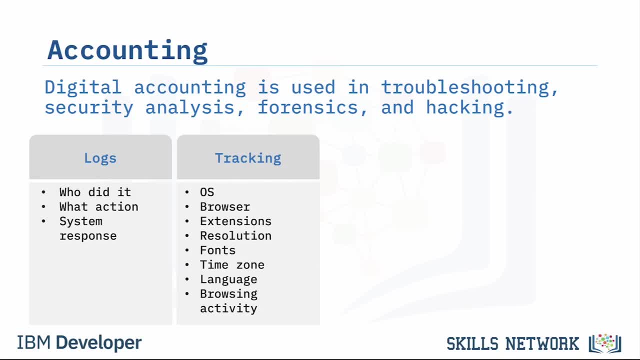 installed fonts, time zone, language and how long you spent on a site and what you did there. Cookies: A cookie is code used to track, personalize and save information about your browsing session. Cookies can also be used to ban you from. 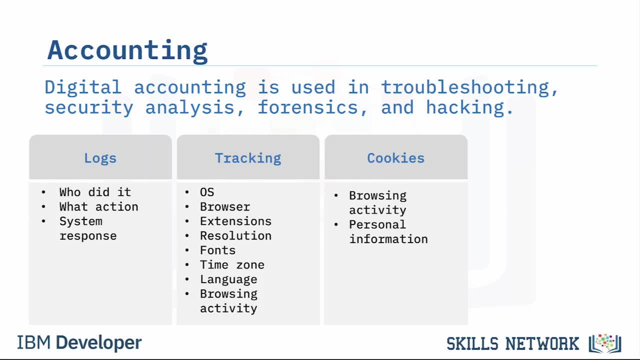 a website if you've violated any of its conditions for use. Browsing history. Browsing history is a list of recently visited websites. Anyone with access to your device can see what sites you visited. Attackers use browsing history to learn where they might impersonate their victims, and companies use it to see which sites you 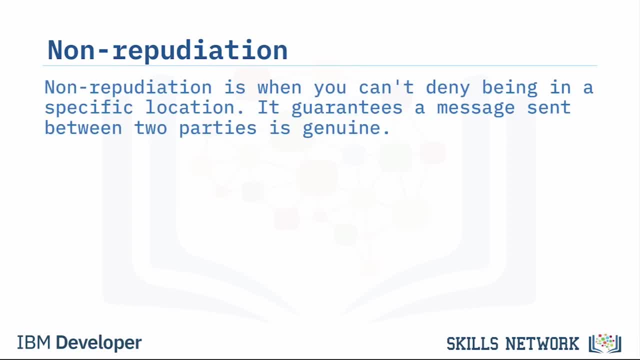 go to on your work computer Non-repudiation. Non-repudiation is when you can't deny being in a specific location. It It guarantees that a message sent between two parties is genuine, like a digital signature. It includes video clear recordings of a person entering, leaving or occupying a space. 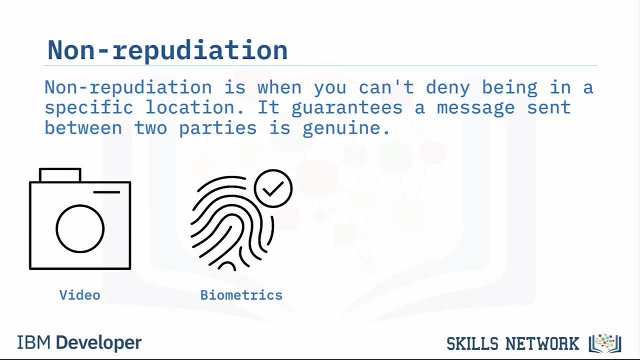 Biometrics, fingerprint or iris scans can confirm whether a person physically accessed a device, network or area Signature: When a signature is used in conjunction with a hardware token, it becomes a digital signature. This authenticates the signer And Receipt. A digital receipt proves that a message was. 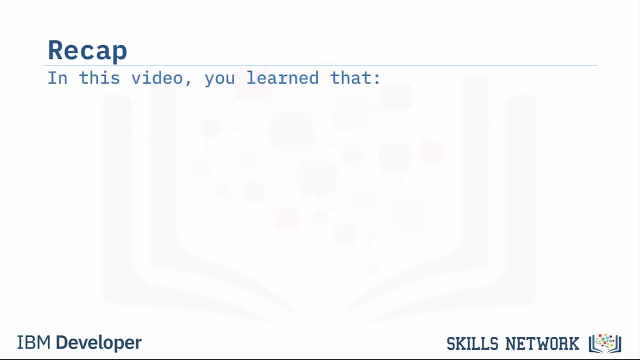 sent from one party to another. In this video, you learned that Role-Based Access Control, or RBAC, uses network groups with different permissions levels. The methods of authentication are single-factor, two-factor and multi-factor. Authentication factors are something you know, something you have, something you are and